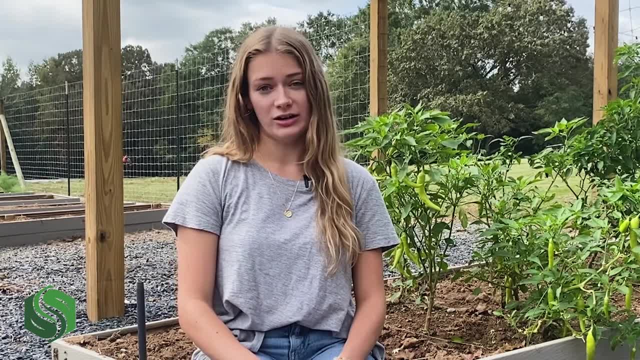 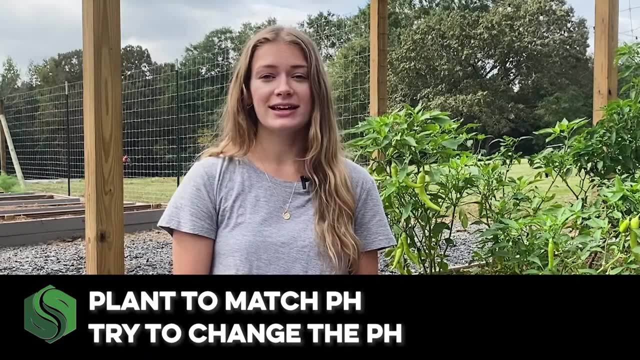 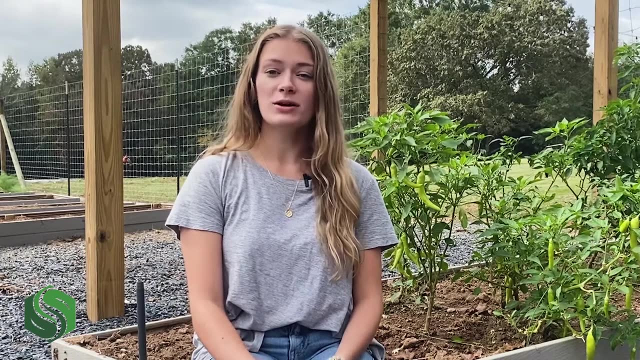 have two options when it comes to soil pH in your garden or landscaping Plant: to match pH or try to change the pH. No matter which route you take, it's best to start by knowing your soil's pH level. You can test soil pH by buying a test kit at a garden center or 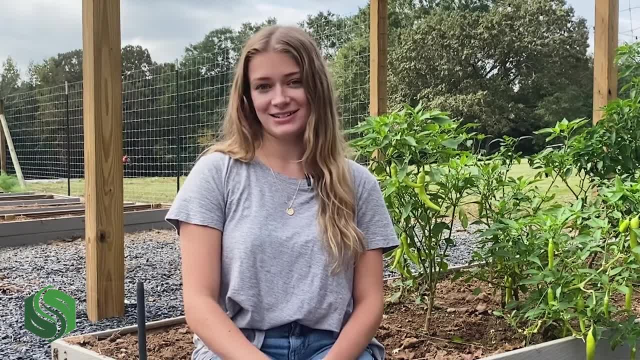 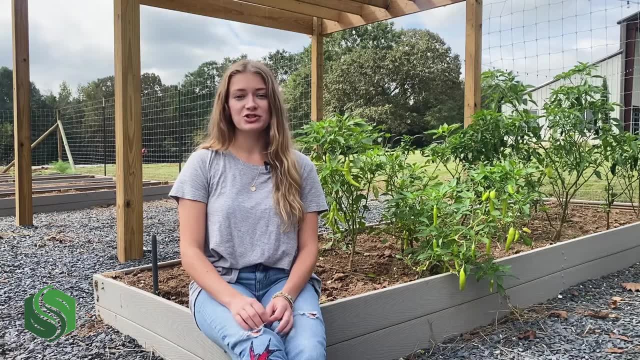 taking a sample to your county extension agent for them to test. If you've tested your soil pH and don't really want to mess around with changing it, make sure to research the plants you're considering And check to see if they're compatible with your soil's pH level. 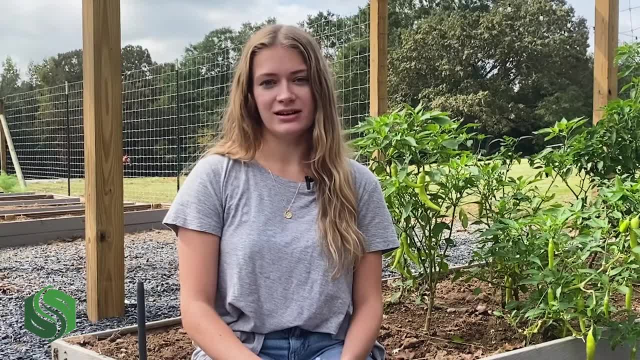 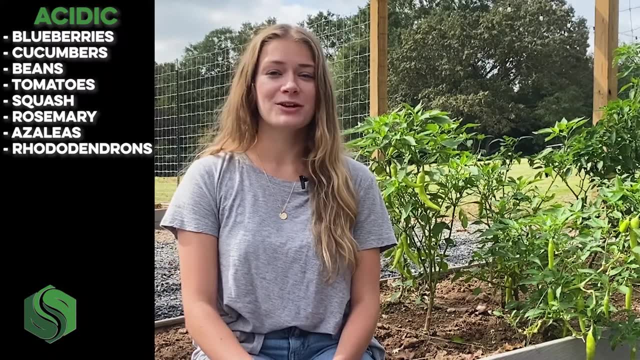 Plants that prefer acidic soil have different ranges of ideal acidity, but some examples are blueberries, cucumbers, beans, tomatoes, squash, rosemary, azaleas and rhododendrons. Plants that prefer alkaline soil also have different ranges, but include okra beets. cabbage, zinnias, lavender and hydrangeas. If you're still not really sure, it's safest to go with a soil pH value between 6 and 7.. If you're still not really sure, it's safest to go with a soil pH value between 6 and 7.. 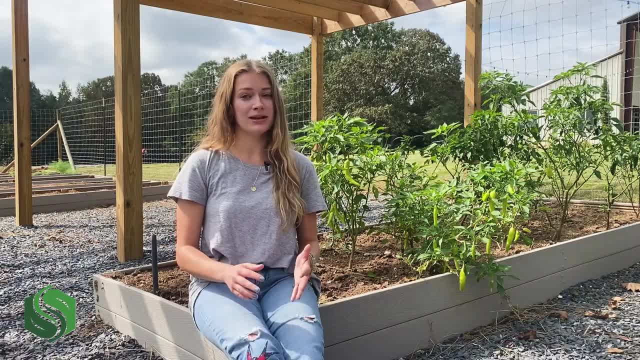 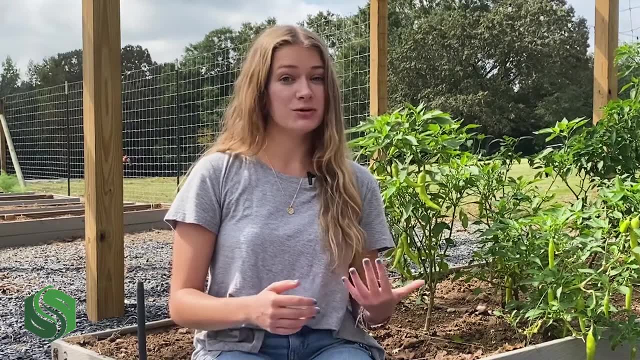 If you're still not really sure, it's safest to go with a soil pH value between 6 and 7.. In this range most nutrients essential to plant growth can be readily available. So let's say you're really set on growing a plant that prefers sour soil, but your soil 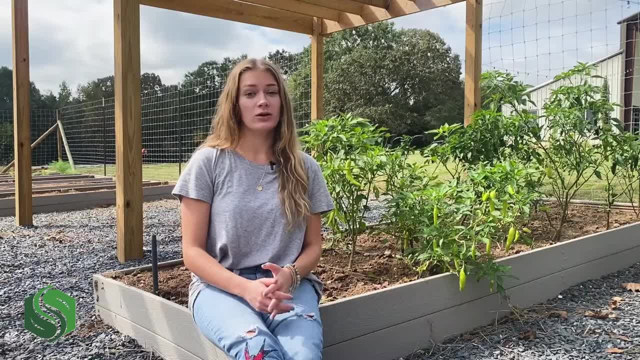 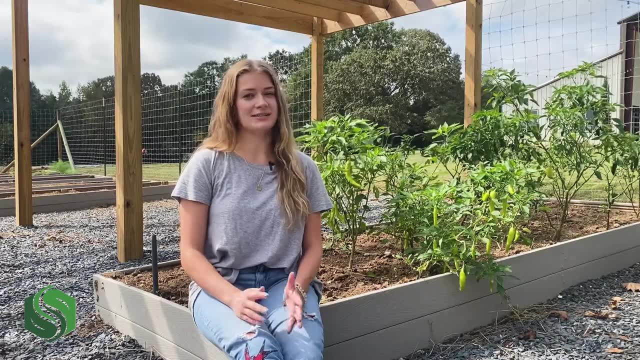 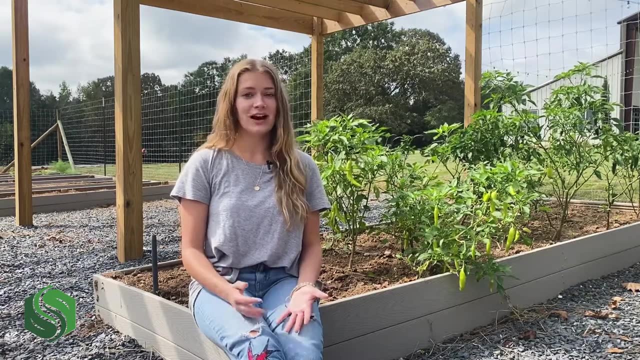 is pretty sweet. You can increase the acidity of your soil or decrease the pH by adding sulfur. Sulfur for soil can be bought at garden stores, but it has a catch. Sulfur converts to sulfuric acid with the help of bacteria in the soil, but this takes time, depending on factors. 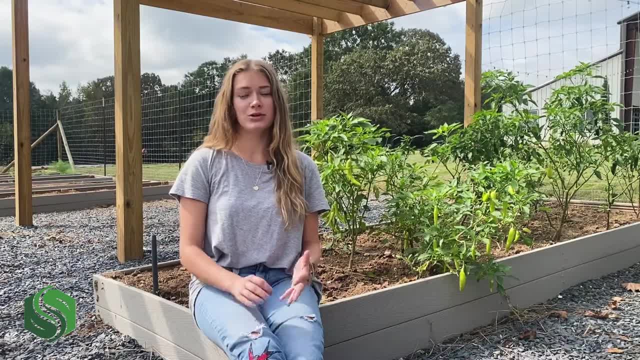 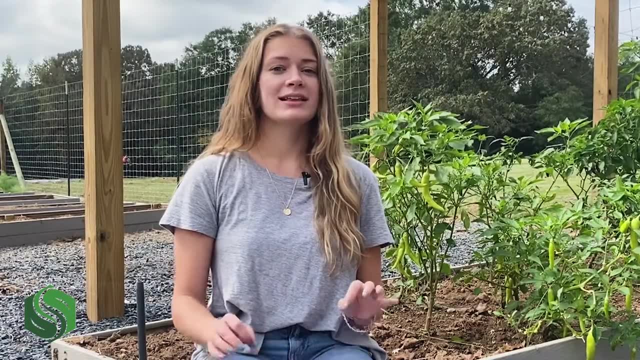 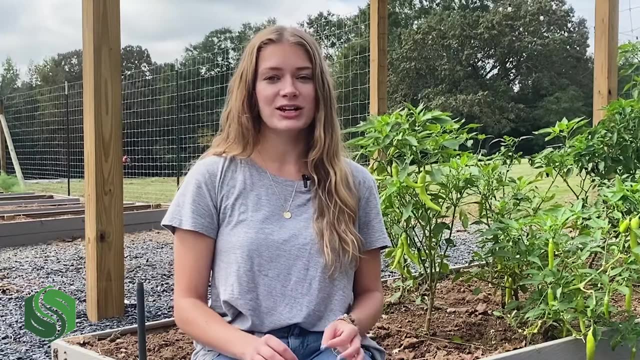 like the presence of bacteria, texture of the soil and moisture levels. This could take months if conditions are not ideal. On the other hand, if you want to make your soil less acidic because you have your heart set on growing a sweet, soil-loving plant, there are ways to increase pH levels in soil. 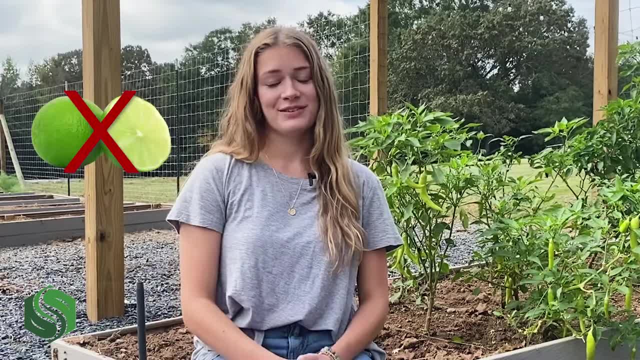 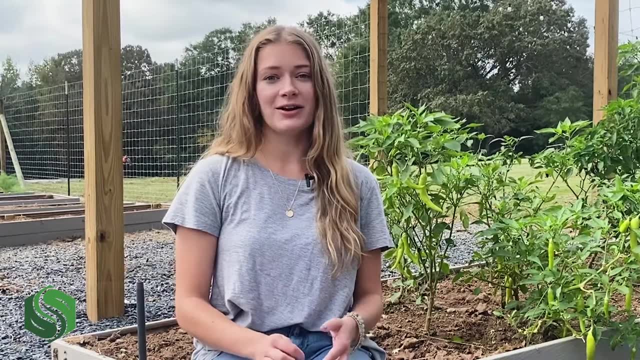 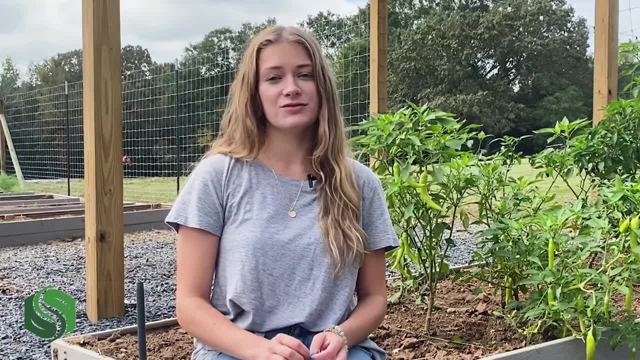 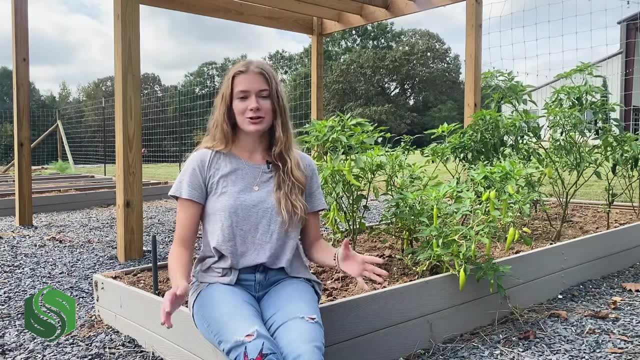 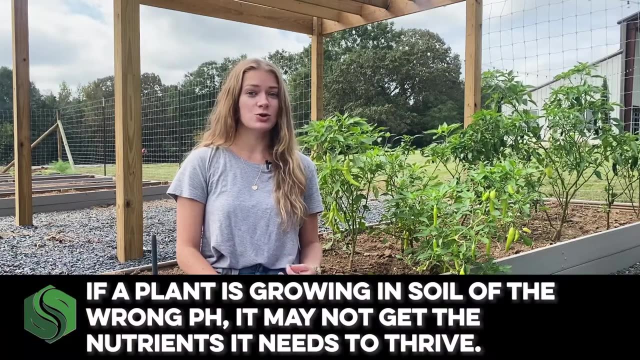 This can also be purchased at home at homecom. This can also be purchased at home at homecom. So why go through all this effort and even consider soil pH? Soil pH has a big impact on the solubility of minerals and nutrients. If a plant is growing in soil of the wrong.